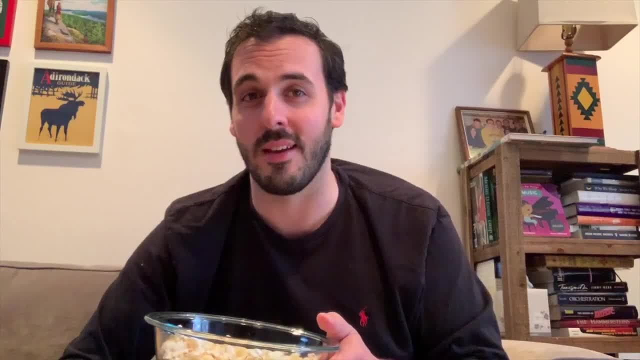 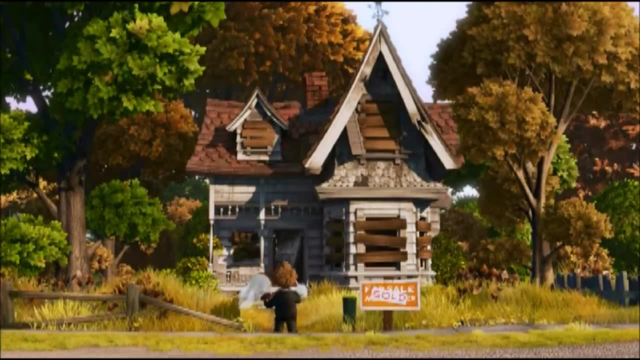 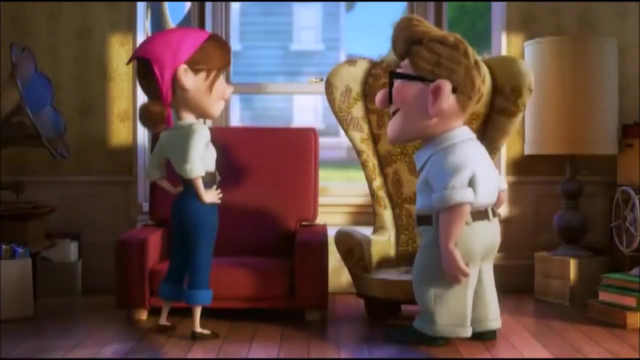 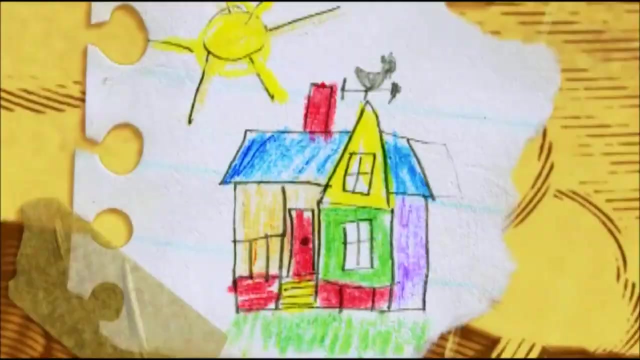 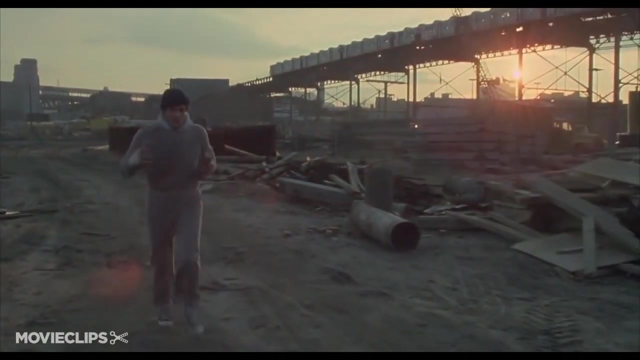 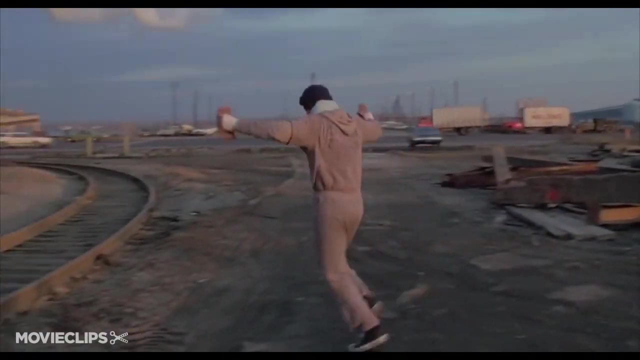 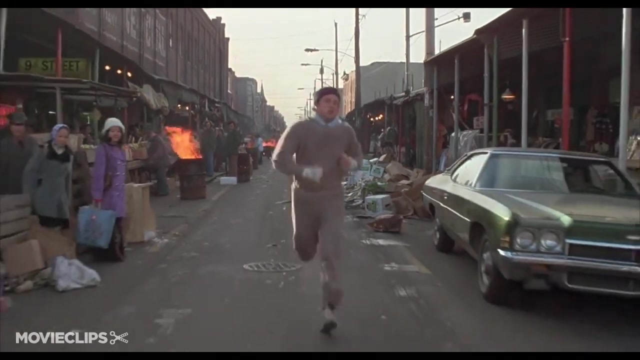 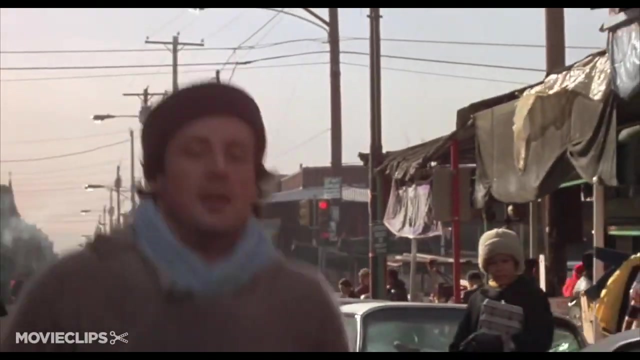 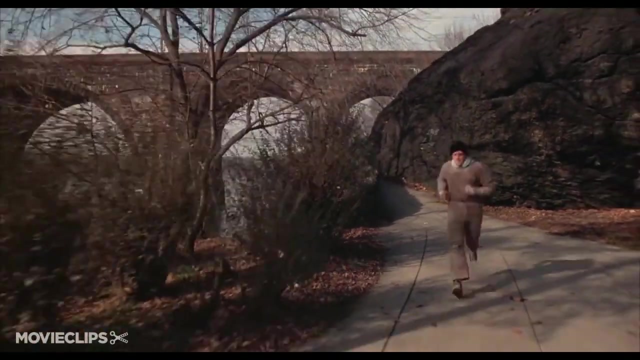 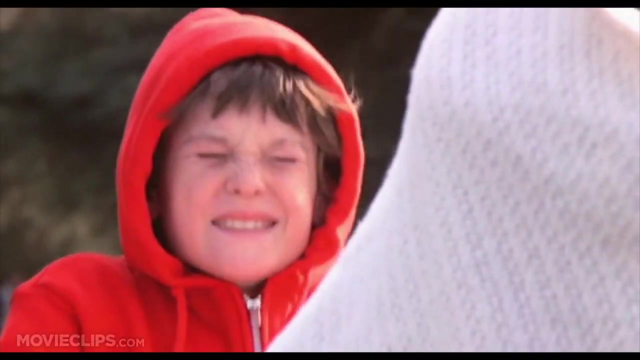 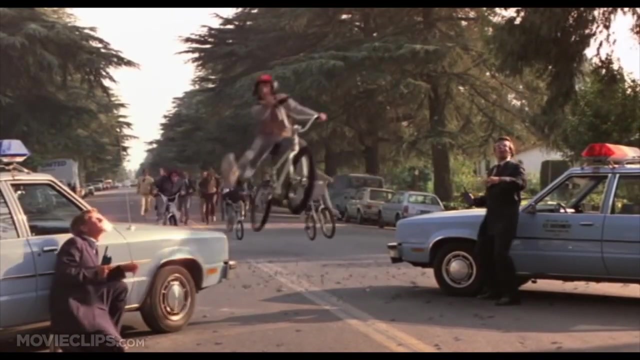 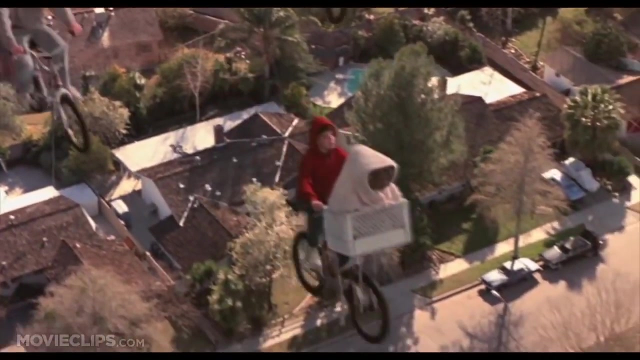 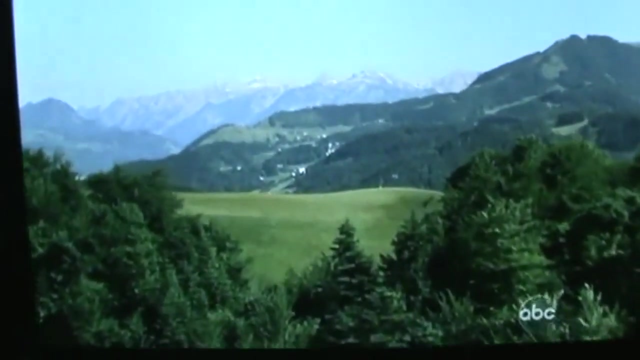 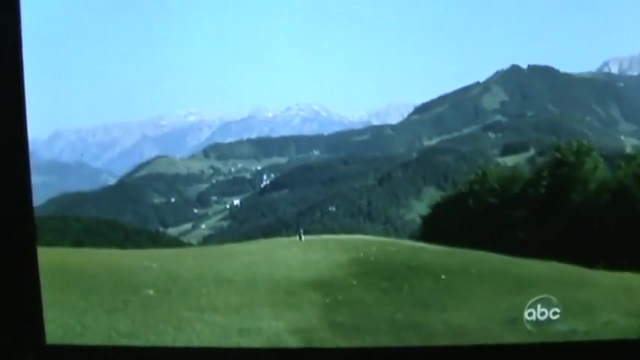 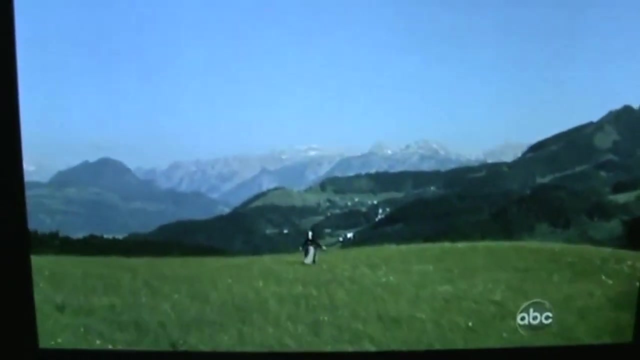 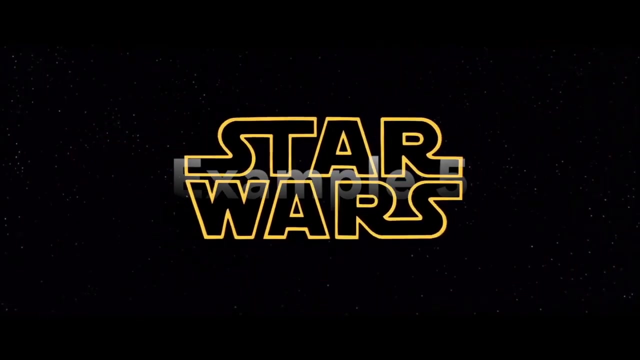 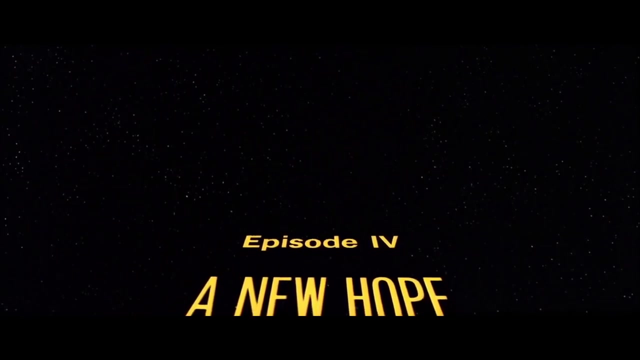 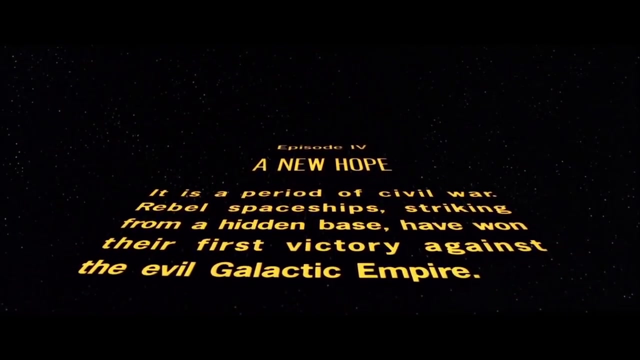 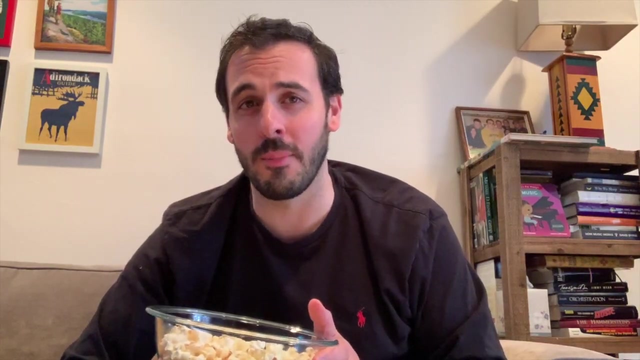 but I've swapped out the music and I've put the wrong music in. Let's check them out. Let's check them out. Here we go, Here we go, Here we go. Well, now that you've seen those clips with the wrong music, 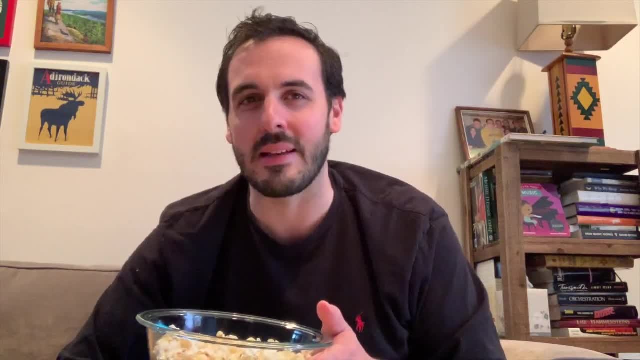 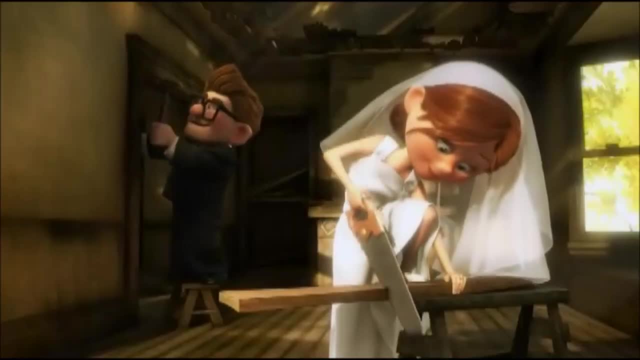 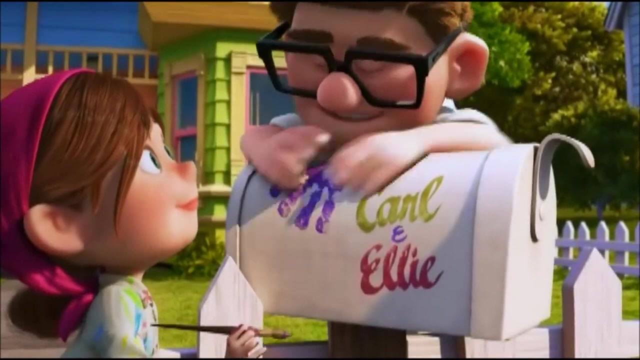 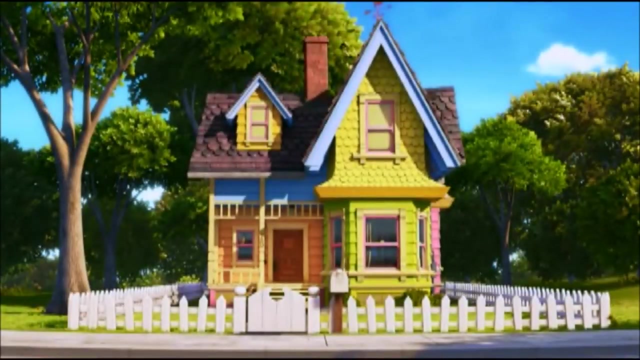 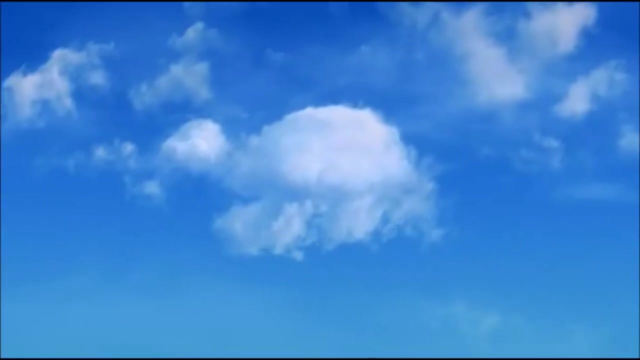 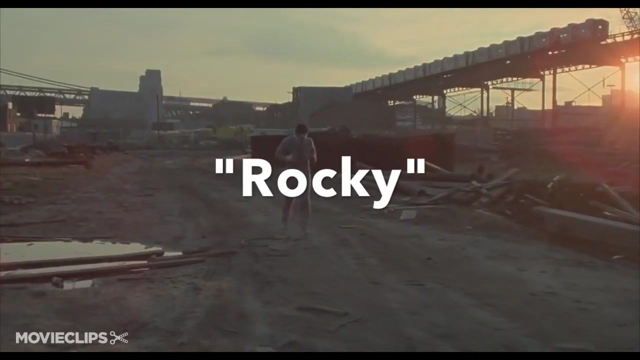 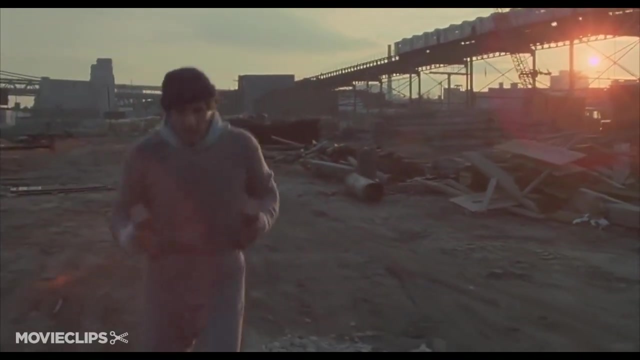 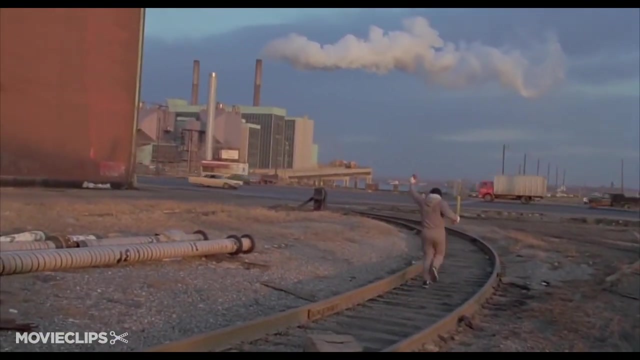 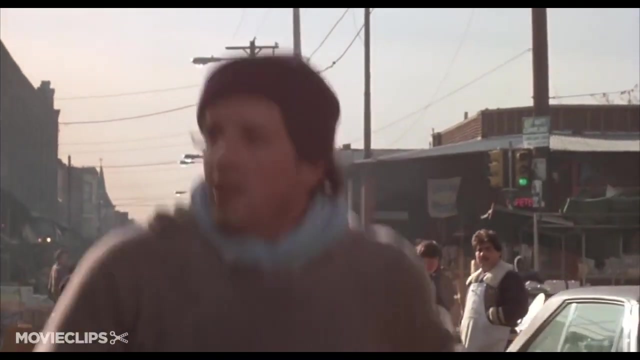 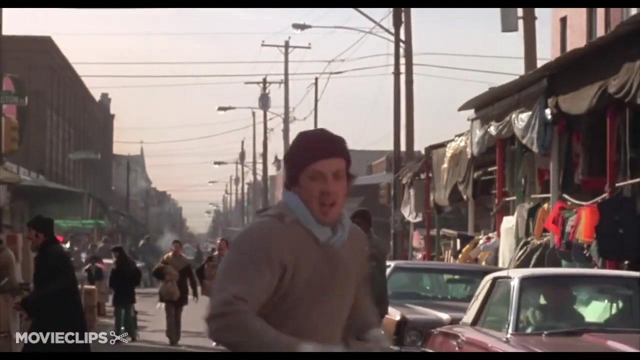 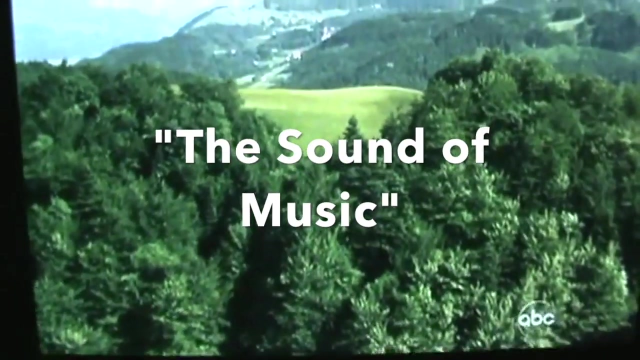 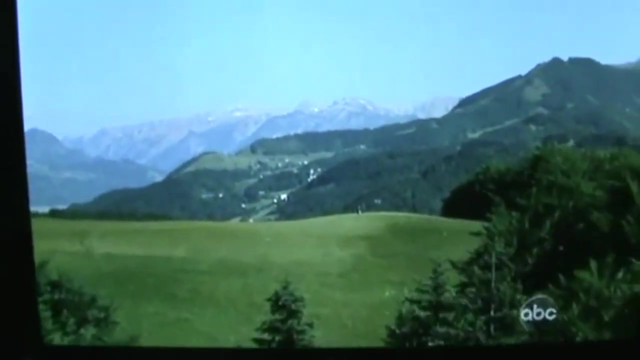 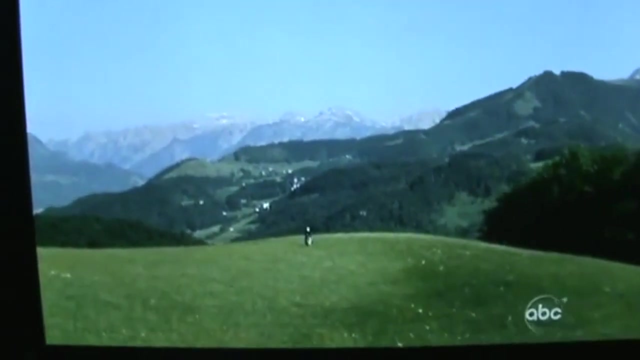 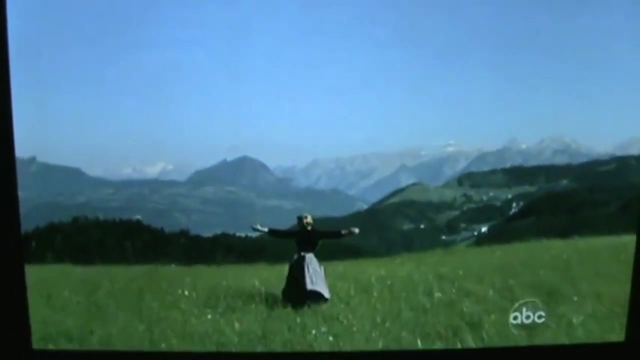 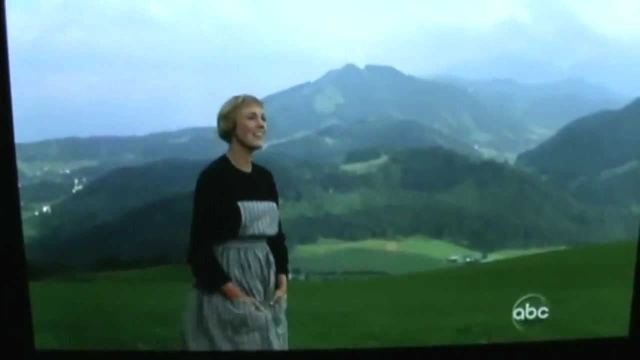 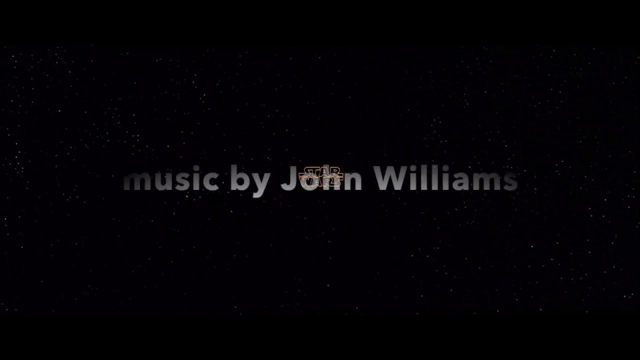 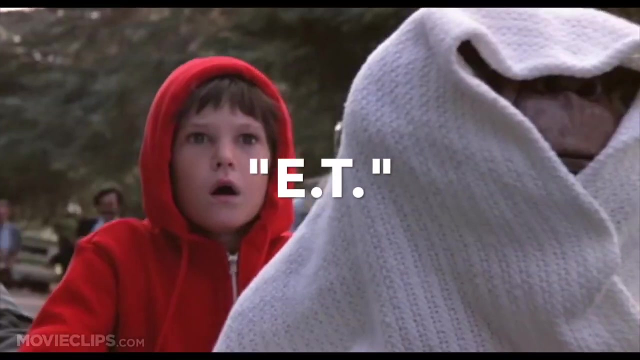 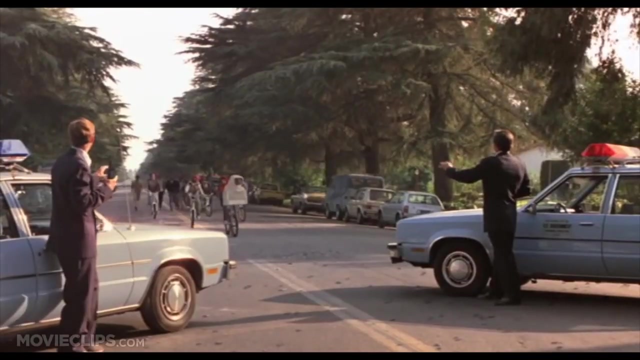 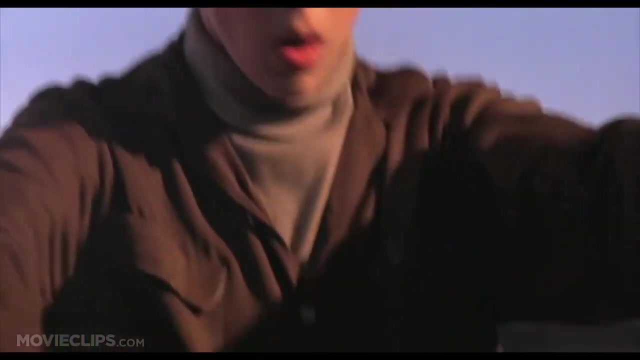 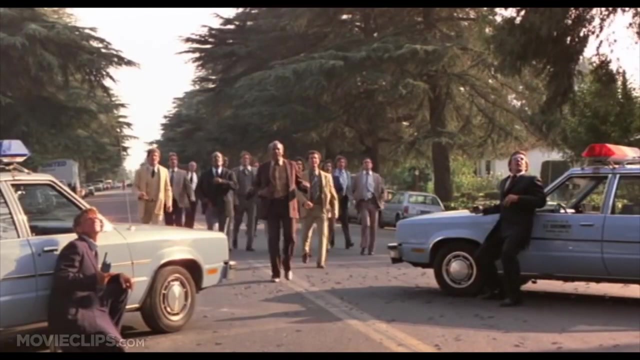 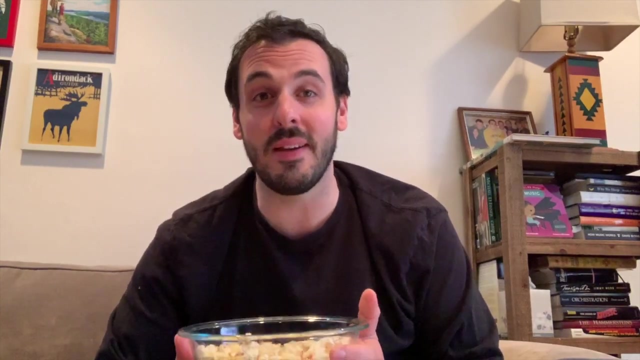 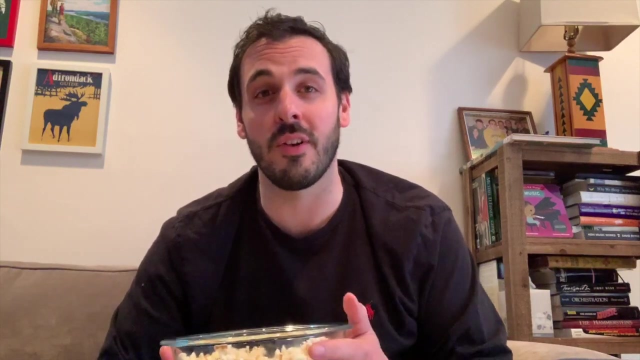 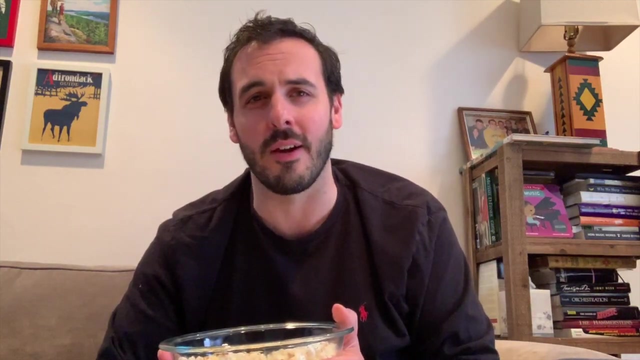 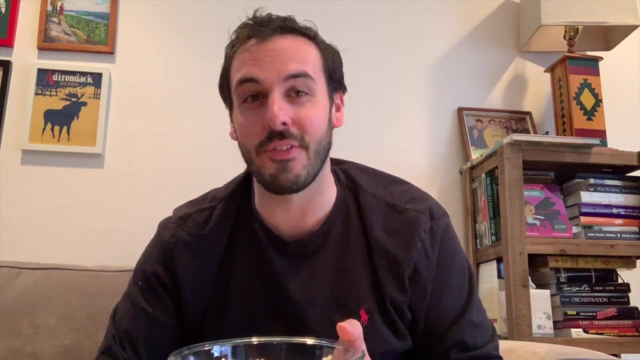